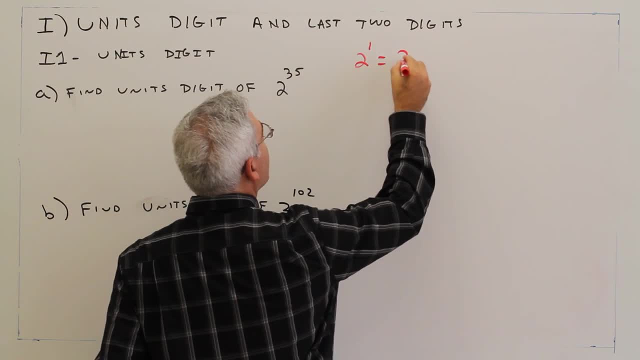 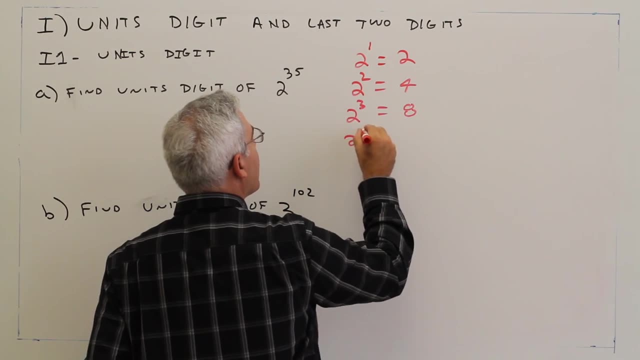 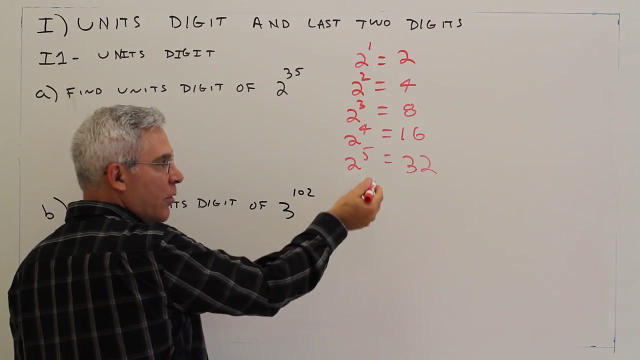 So 2 to the 1 is 2,, 2 squared is 4,, 2 cubed is 8,, 2 to the 4th is 16,, 2 to the 5th is 32, and the pattern is going to continue in cycles of 4.. 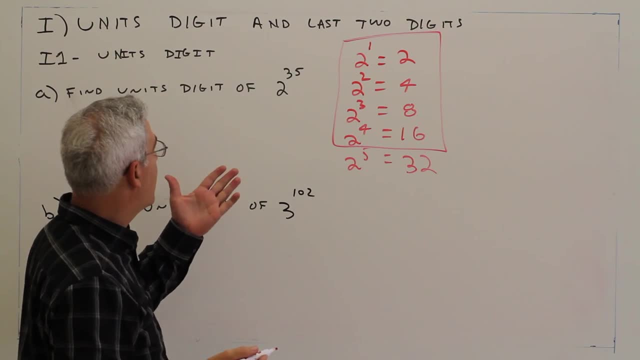 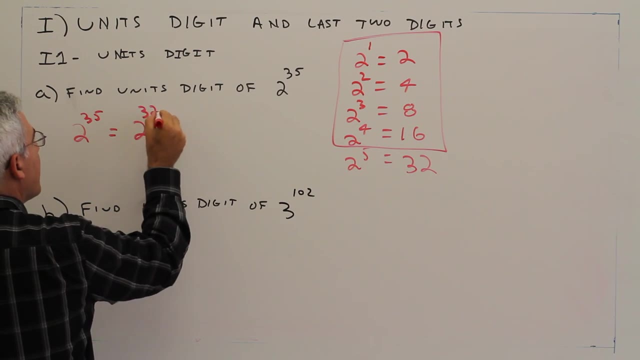 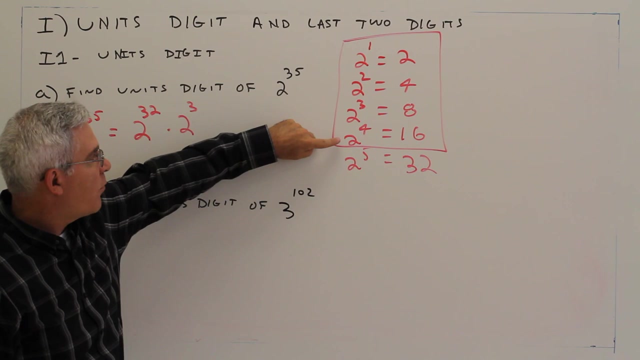 So what I do. there's two different ways of doing this, so you could do it this way: 2 to the 35th is the same as 2 to the 32nd, times 2 cubed, And 2 to the 32nd is pretty much going to get you here. it's a multiple of 4, and then I've got to add 3, 1,, 2, 3.. 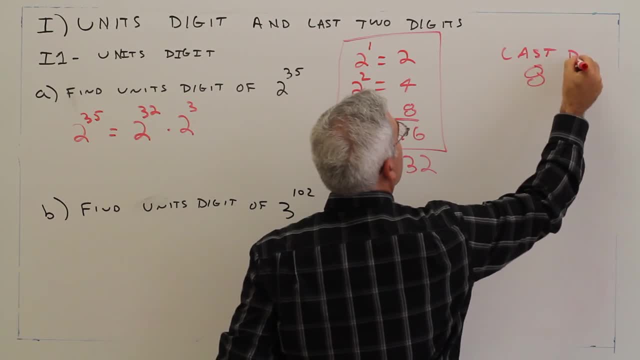 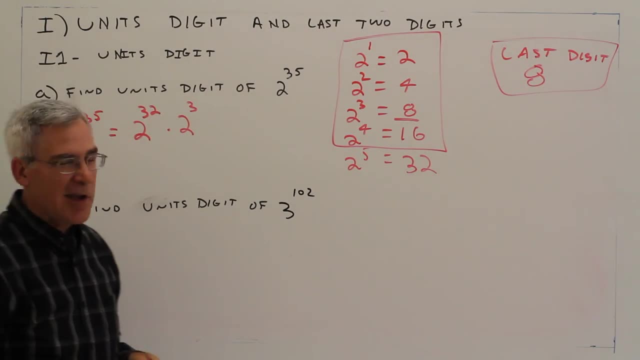 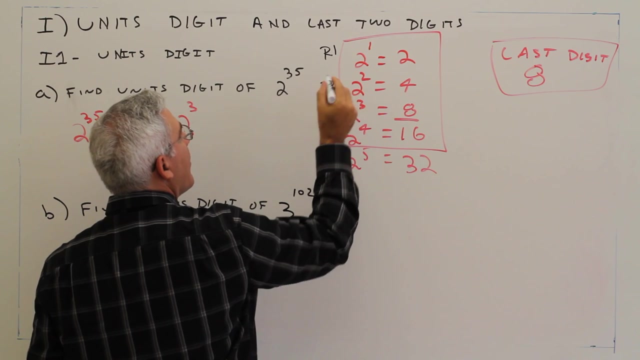 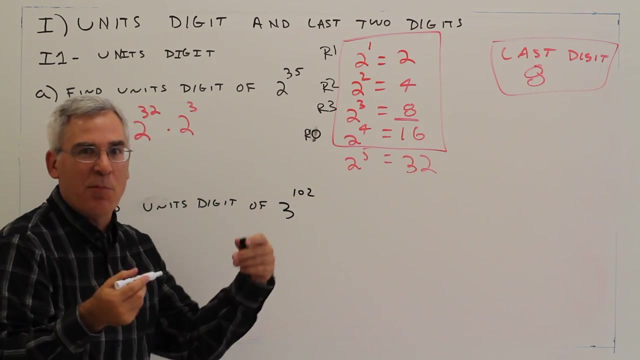 So you'd get a last digit of 8.. Another way of doing this is to find the units digit of 8.. Another way of doing it is dividing and looking in terms of remainders, So thinking this is like a remainder 1, this is a remainder 2, this is a remainder 3, this is a remainder 4, really a remainder 0, because it's multiples of 4.. 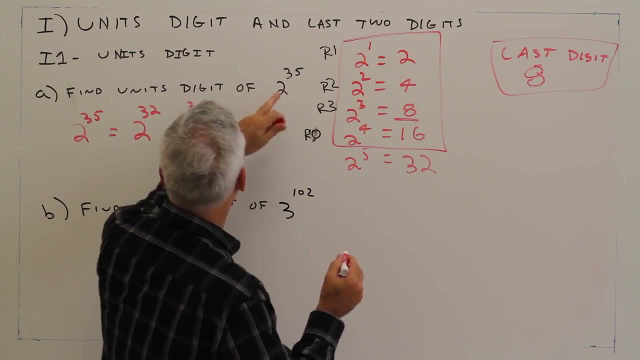 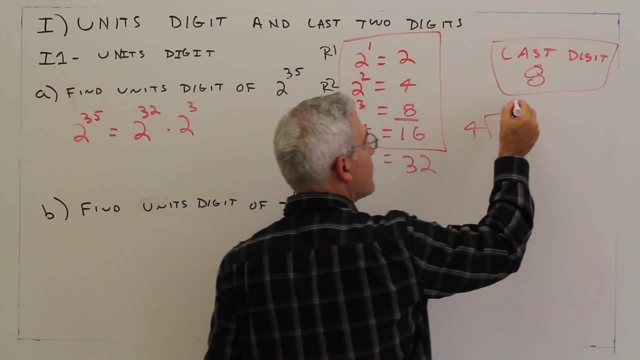 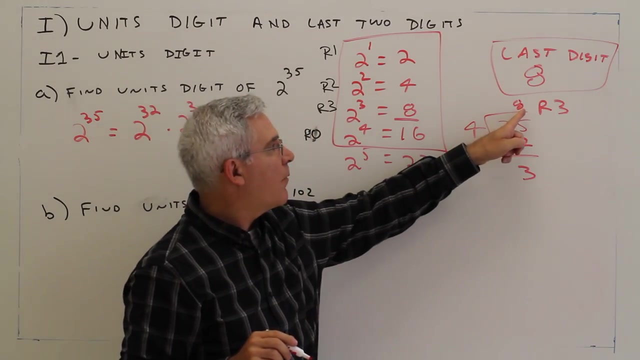 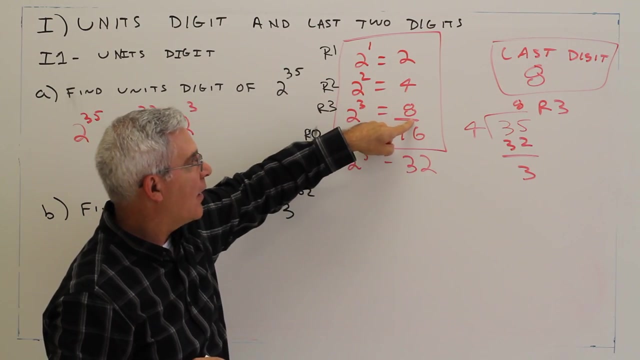 Alright. so what we could have done is done: 35 divided by 4.. And the answer is 8 remainder 3, just a coincidence that that 8 is the same as that. So remainder 3, going to remainder 3 and getting an 8.. 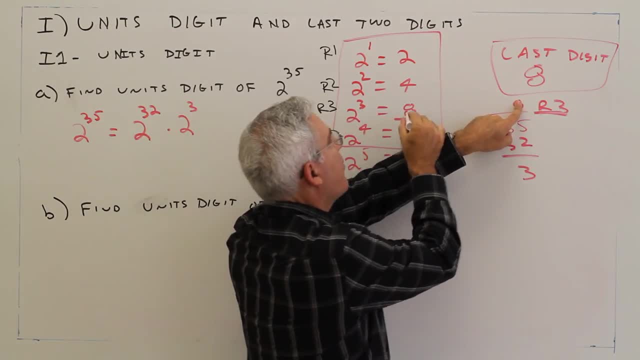 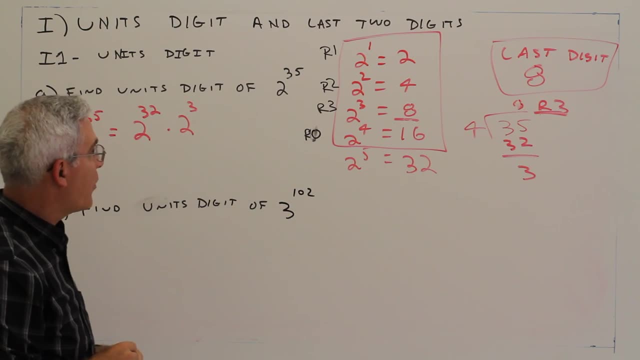 Again, it's this remainder 3, and this remainder 3. there that's giving you the answer. Okay, next problem: 3 to the 102.. Again, we'll look for a pattern. So 3 to the 1st, 3 squared, etc. 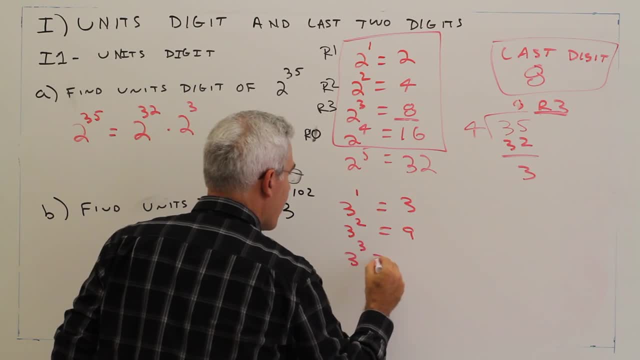 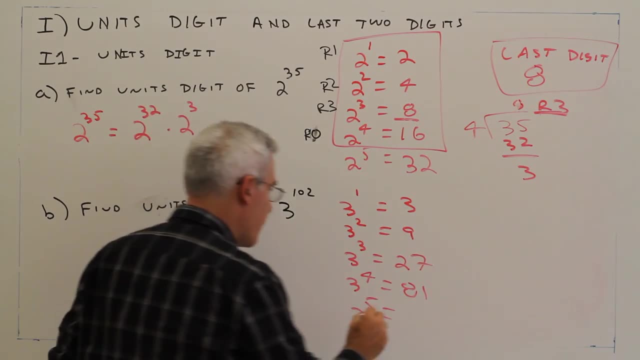 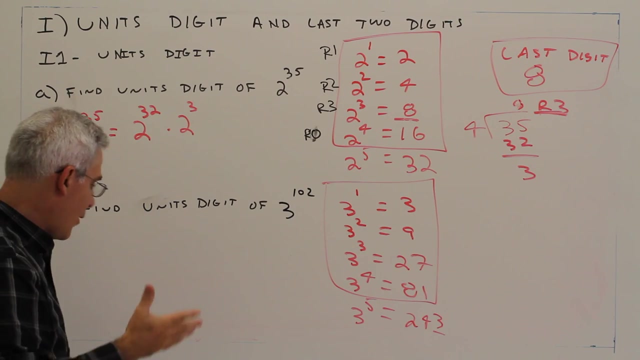 The 1st is 3,. 3 squared is 9,, 3 cubed is 27,. 3 to the 4th is 81,, 3 to the 5th is 243.. Again, we have a cycle of 4, so I'll just do it the division way.